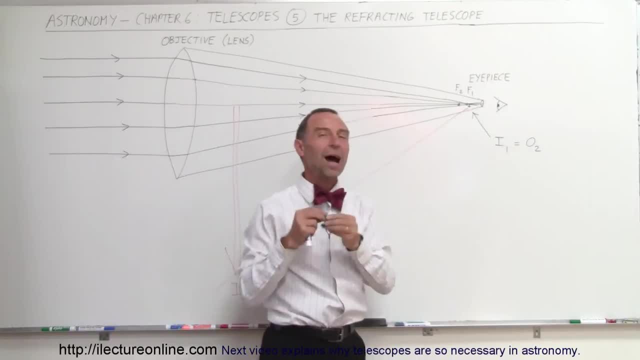 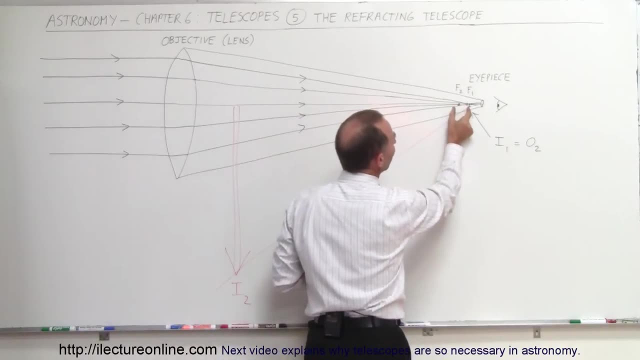 see here on the controller, you are looking at the focal point of that first lens. so there's your first image which now becomes the object of the second lens. so that image there now acts like an object to the second lens, since that object is within the focal length or the, or closer to the. 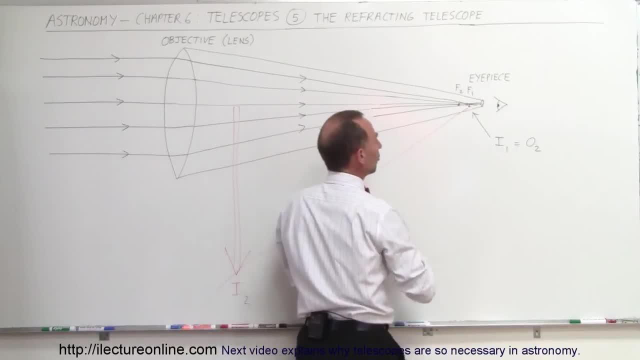 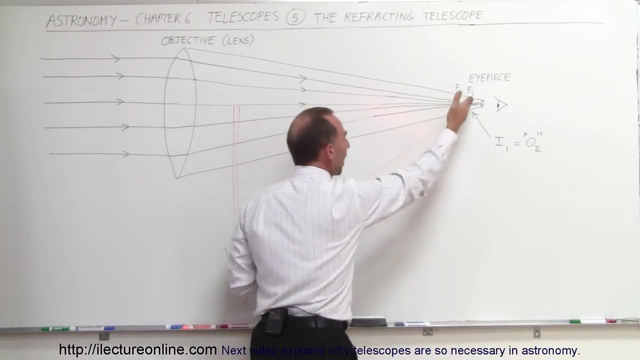 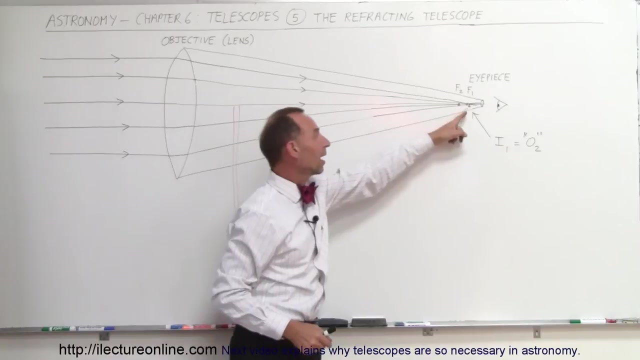 lens on the focal point of that second lens, you will end up with a virtual image of that object. so this is basically an object or the image of the first lens that acts as the object of the second lens, and it'll be upside down, because the first image is upside down. that means 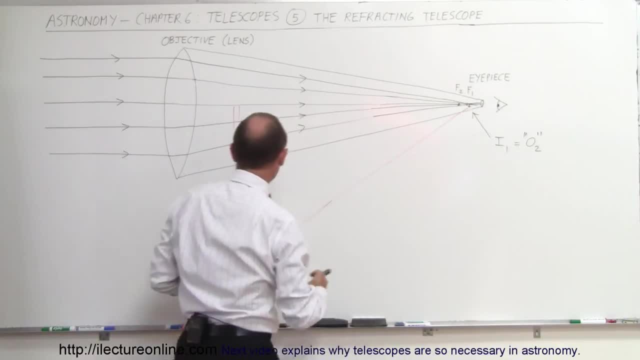 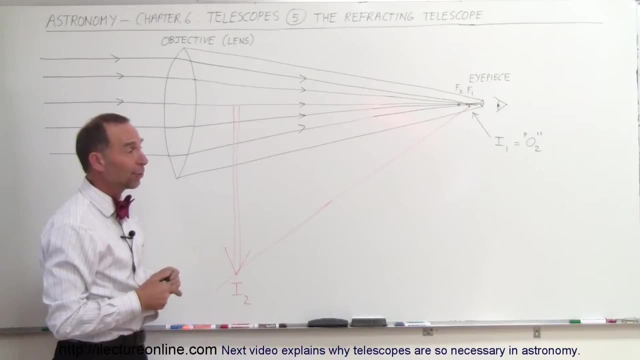 the object of the second lens will be upside down as well, which will form an upside down virtual image. so when we look through a telescope, we actually see everything upside down, and if you want to see what it looks like right side up, you just simply have to turn the picture and turn 180 degrees around. but notice, 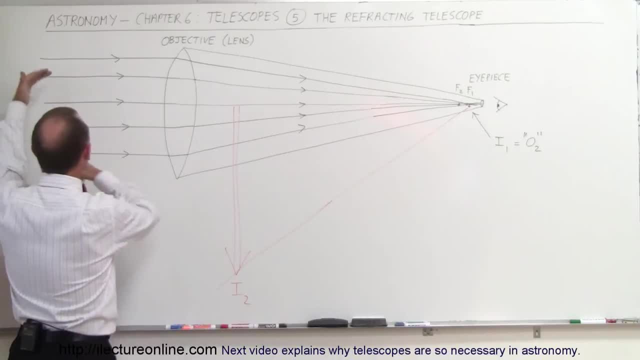 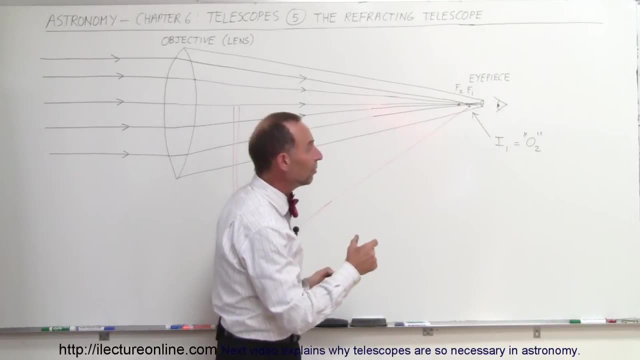 how it uses the principle of the two lenses. for faraway objects. the image will form very close to the focal point, just past the focal point for the second lens, since the object is inside the focal point, as we call it, closer to the lens. on the focal point of the second lens, a virtual image will be formed. 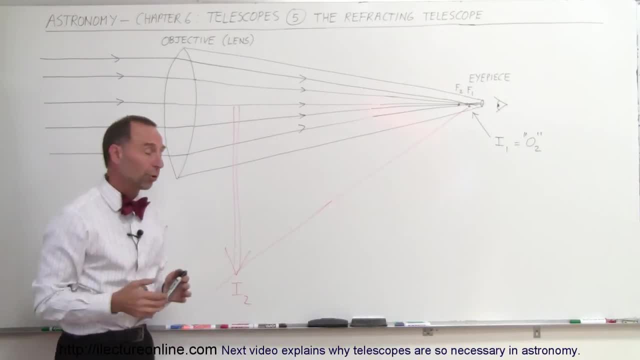 making the final image that the astronomer or the observer will see, and it's very much enlarged, as you can see. now, what would be the magnification, as we call it? how much bigger is the final image compared to the original object? well, it turns out that the magnification is much bigger than the original object. 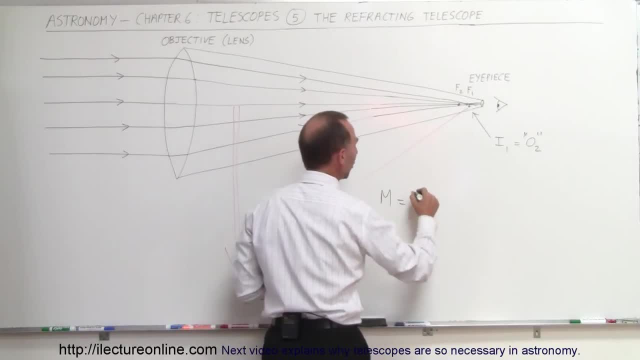 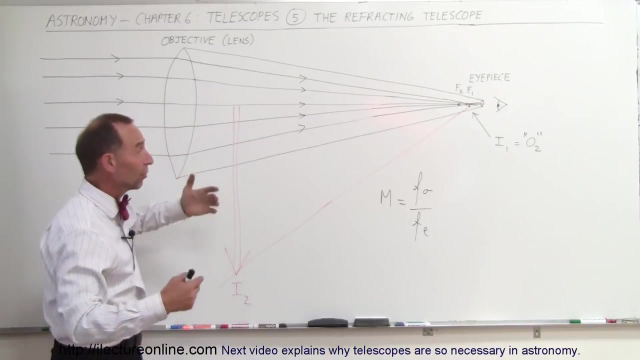 magnification. and for magnification is simply the ratio of the focal length of the objective. so we called the focal length of the objective divided by the focal length of the eyepiece. so typically the focal length of the objective can be 50 centimeters, 100 centimeters, you know, three feet four. 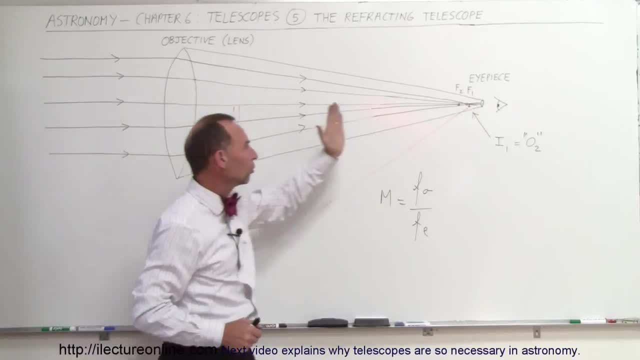 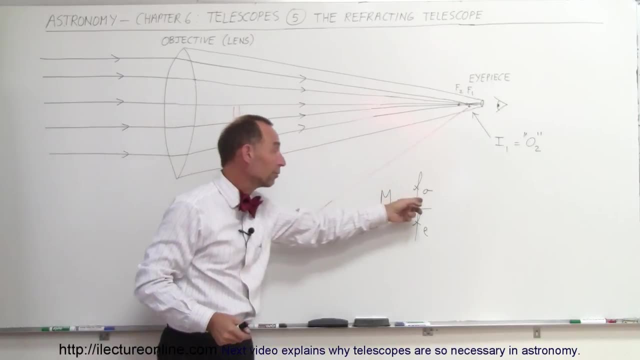 feet five feet. however long your telescope is, it's basically almost the length of the telescope. if you have a really long telescope that's one hundred feet or two hundred feet long, then of course the focal length of the objective is a very large focal length and the focal length of the eyepiece is usually very small. so, for example, 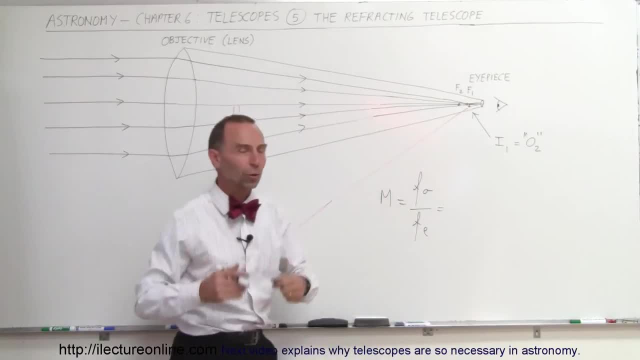 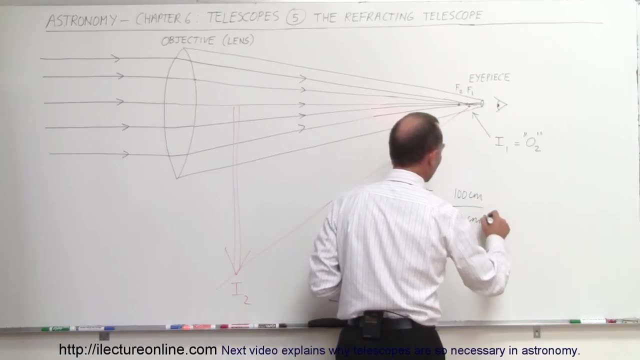 let's say, for a typical telescope that you can buy at the local store, you may say that the focal length of the objective is 100 centimeters and the focal length of the eyepiece, let's say, is two centimeters, and then, simply, the magnification is then a ratio of 50 to 1. in other words, all 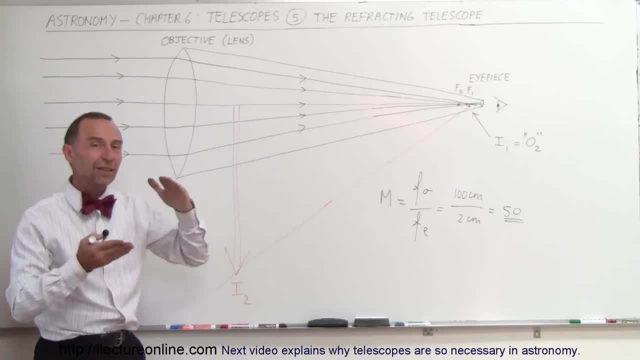 objects that you see through that telescope would then appear 50 times larger, as you would see them with the naked eye. when you're not using a telescope, that's not necessarily the most important factor. most people think: oh, you want a telescope with a very large magnification. 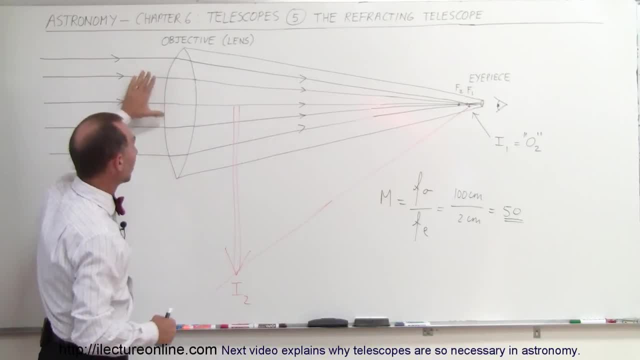 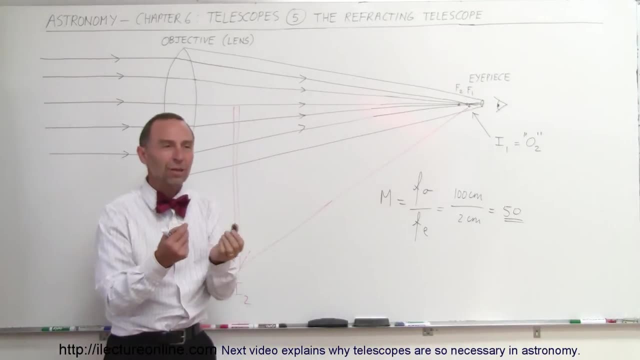 the problem is, if you make it very large but the telescope is relatively small, you can't get enough light into the telescope to make the image visible. the image may be so faint you can't even see it, even though the objects may be. the image that you're looking at may be very large. 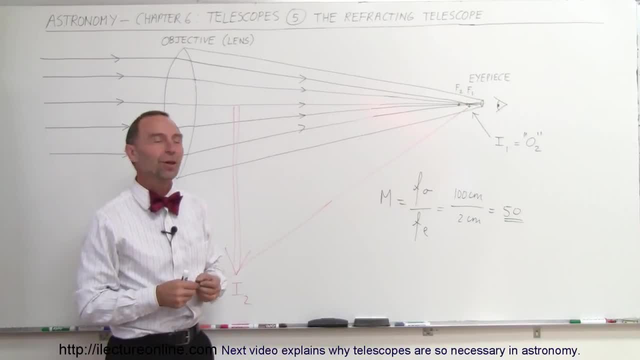 it may not do you much good if it's so faint that you can't see it. so magnification, yes, it's one factor, the telescope- but clarity and resolution and visibility is even more important. so in the next several videos i will show you what's really important. 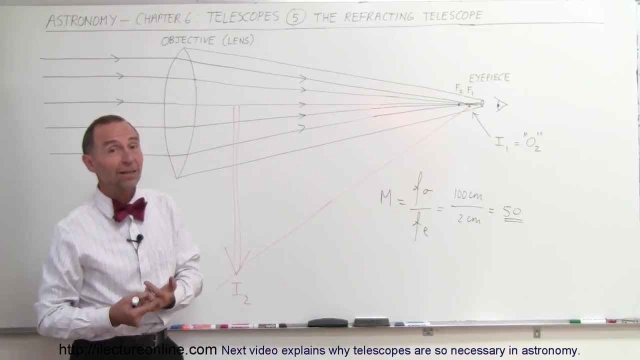 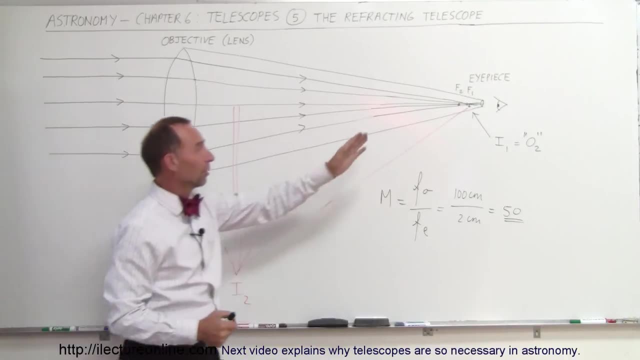 about the telescope and what the most important factors is when you're looking to buy a telescope. so i'll show you that. but the simple fact is two converging lenses: a big one called the objective, a small one called the eyepiece. place them apart in such a way that the focal point just overlap. 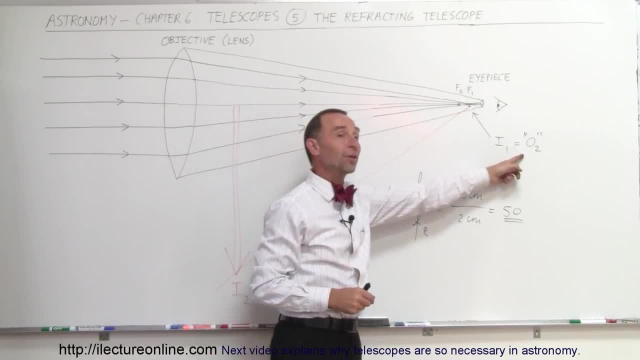 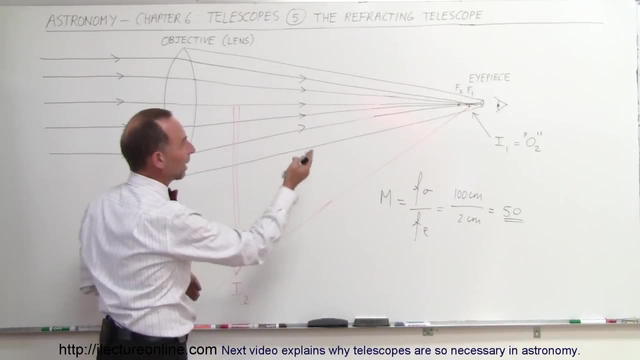 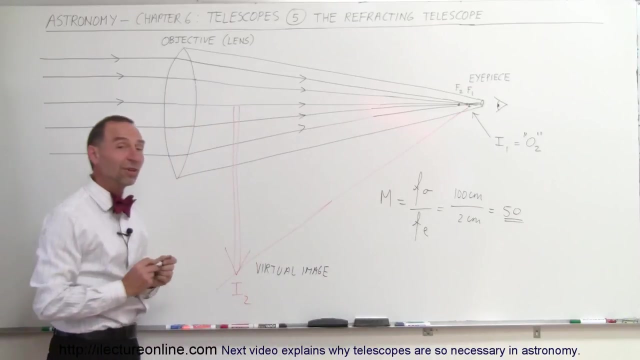 just barely the image of the first lens will become the object of the second lens. that object, since it appears within the focal point of the second lens, will become a very large image. that's virtual, and so make sure we realize that it's a virtual image and it's upside down, and that's what we see. 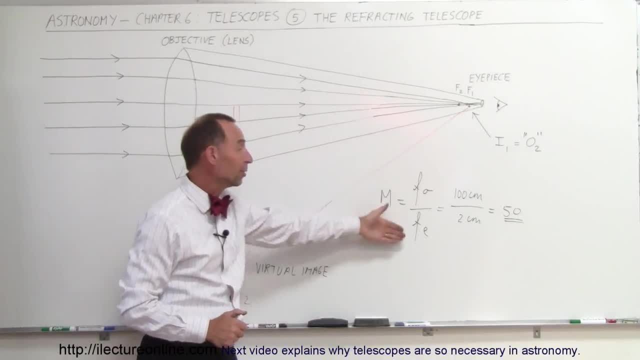 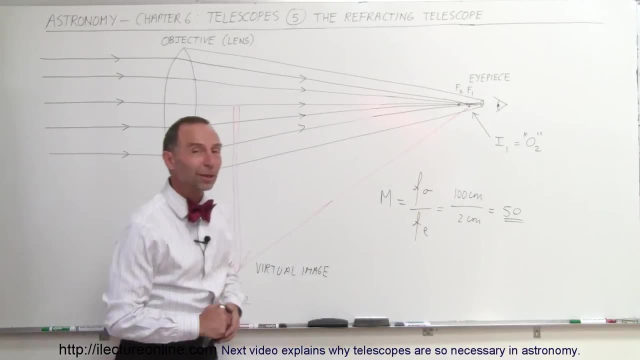 when we look through the telescope and the magnification is simply the ratio of the focal lengths of the large objective lens and the small eyepiece, and usually those are pretty big numbers. that's how we see that. so